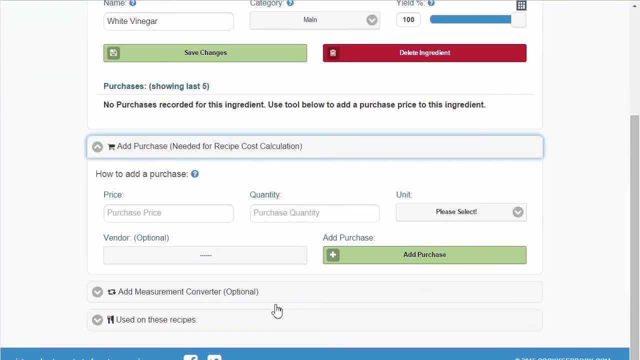 Once in the add purchase section you will have four fields to fill out: price, quantity, unit and vendor. In the price field type: the price you paid for the ingredient without the currency symbol. In the quantity field type: in the number of units you purchased. 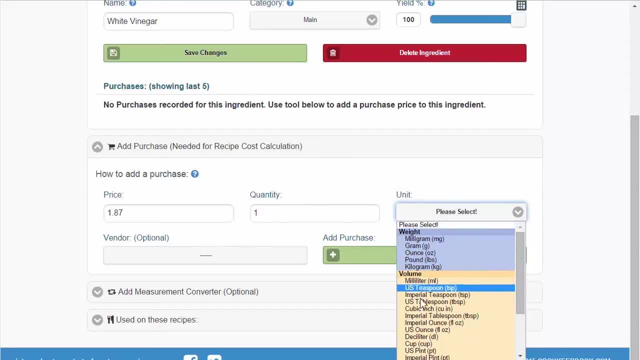 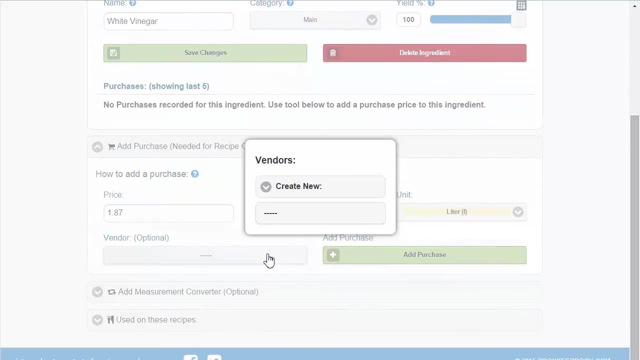 Once you've specified that, select the corresponding unit of measurement for the quantity. You can also specify where you purchased the ingredient using the vendor field. Saved vendors will show beside the purchase price in the ingredient's history. Adding a vendor to the list is easy. 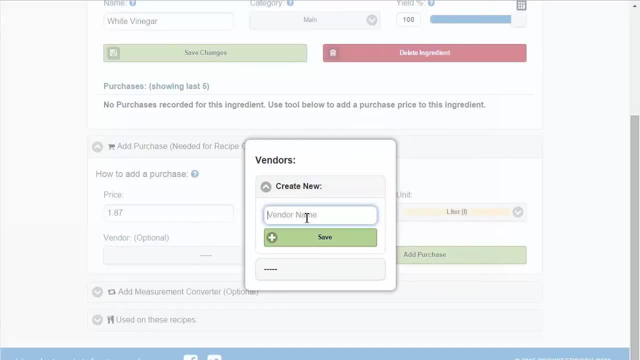 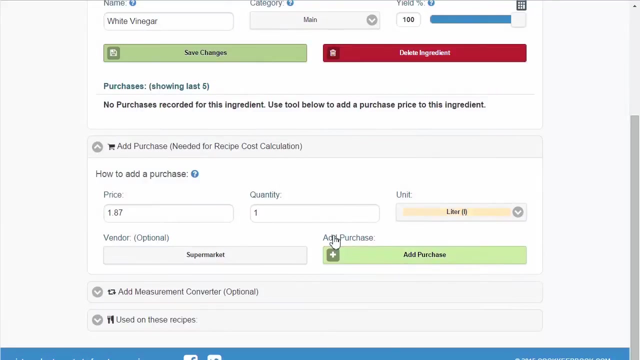 Click create new. in the vendor popup Type in the name of the vendor and press save. It is now available to be selected. You can also edit and remove vendors in this popup window. Once all fields are entered, press the add purchase button to save the purchase. 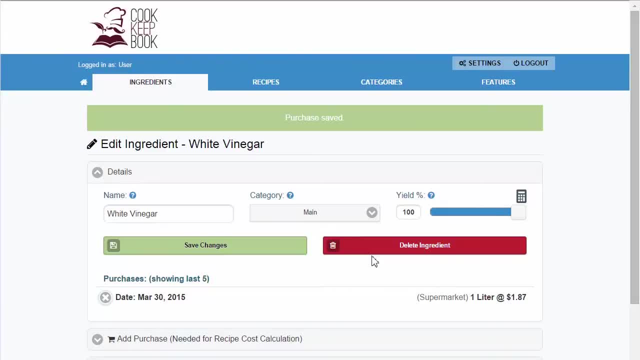 Your purchase entry will now show. in the details section. You can see your last five purchase prices. To remove the purchase entry, click the X button in front of the purchase. This will prompt you to confirm you want to do this. Once confirmed, the purchase will be removed. 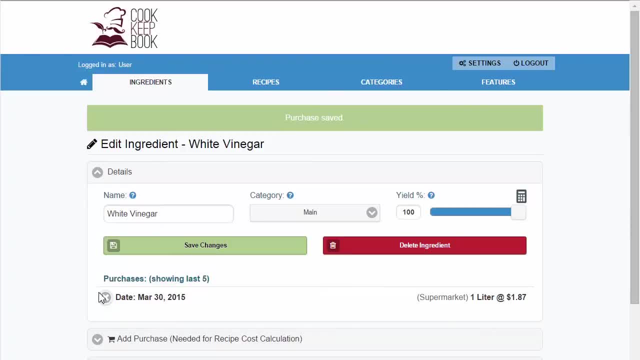 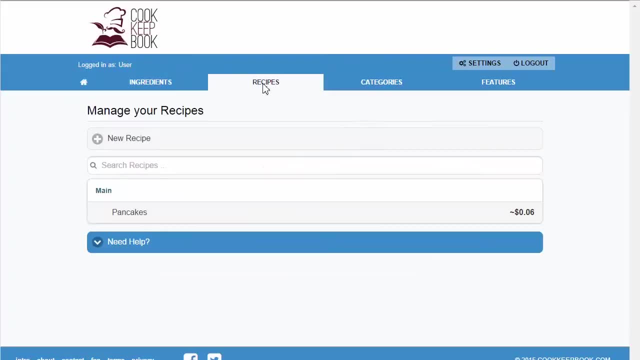 Adding and removing a purchase will update all recipes that have this ingredient in it. Checking our recipe listing again, you will notice that the price of the recipe has been updated. The tilde in front of the cost indicates that not all ingredients could be calculated. 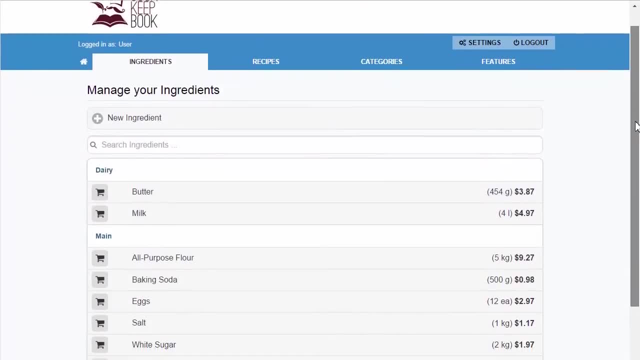 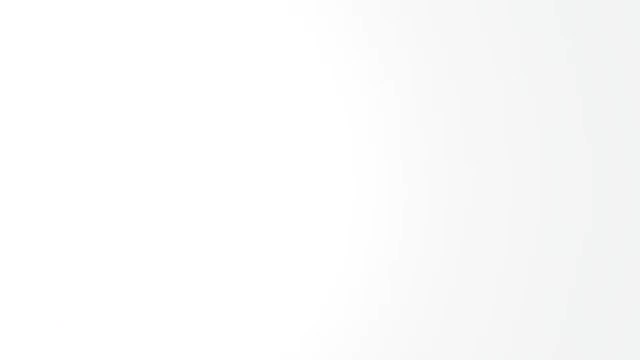 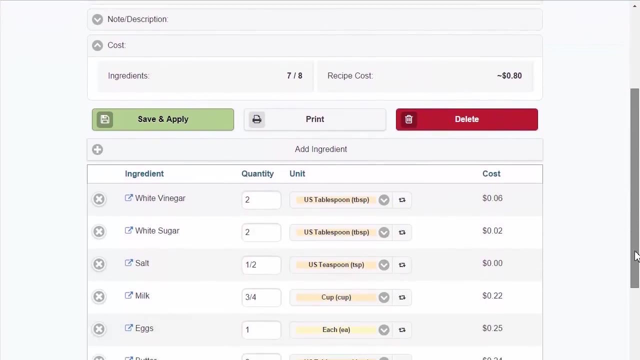 Repeat this process until all ingredients have a purchase price added to them. At times, CookKeepBook still can't calculate the cost of the ingredient because it needs a measurement converter. This happens when the purchase was done in a different measurement type than was put. 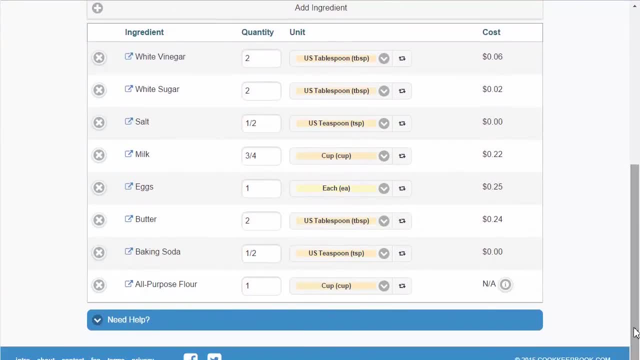 on the recipe, such as weight, volume or count. In this case, flour was purchased in pounds, a weight measurement type, But the rest was added to the list. The recipe called for cups, a volume measurement type. To be able to convert weight to volume, you need to provide a measurement converter between. 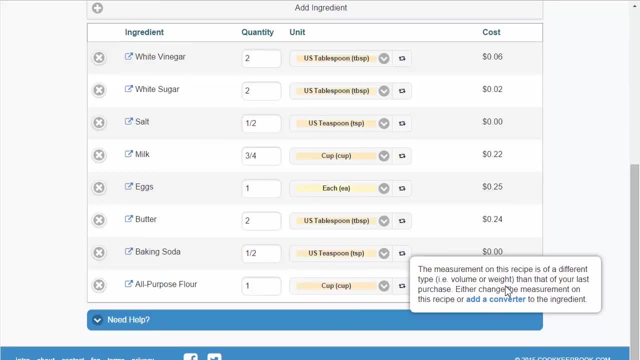 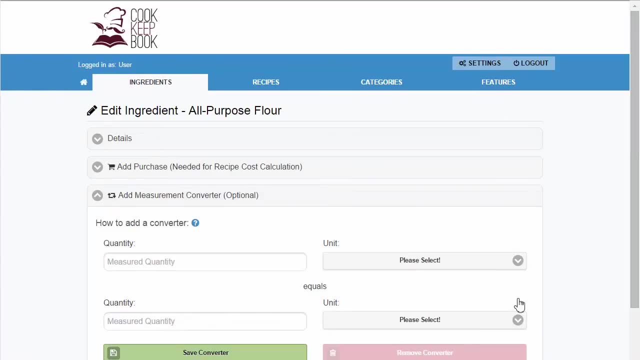 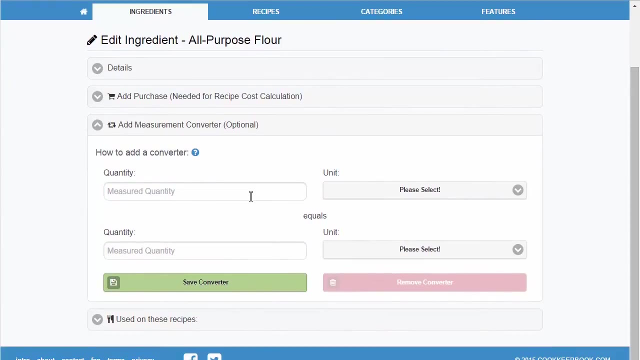 these two types. Click on the link in the information bubble to open the ingredient in a new tab and view the measurement converter section. In the measurement converter section you can enter in the corresponding values for the converter. In our example, one cup of flour.